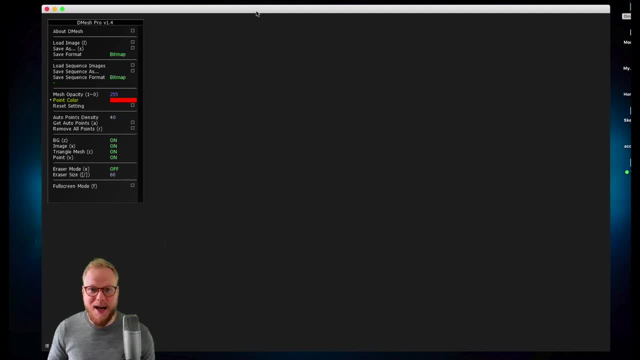 to when I talk to junior designers and they don't know how to make a fancy background. let's say, which would be fractal D mesh? you basically just open bitmap an image and then it fractalize it for you. it makes it much more abstract. Let's say: this is the background I want to play with, for 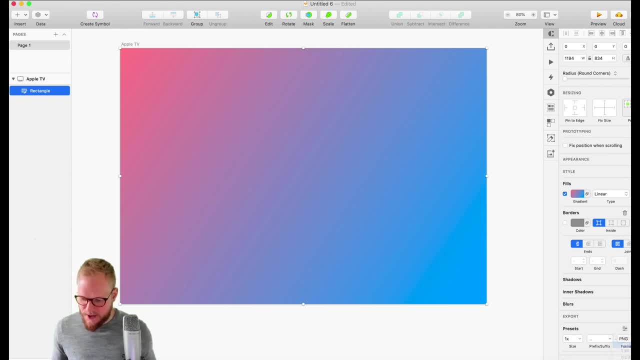 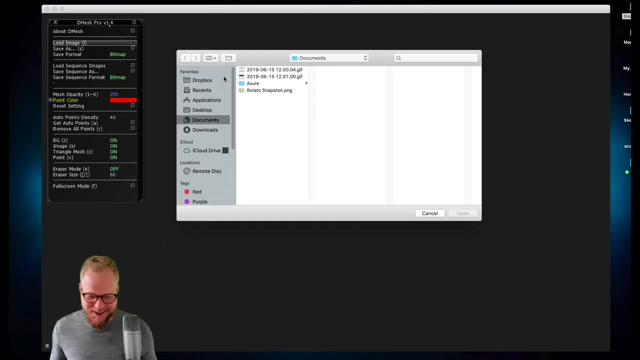 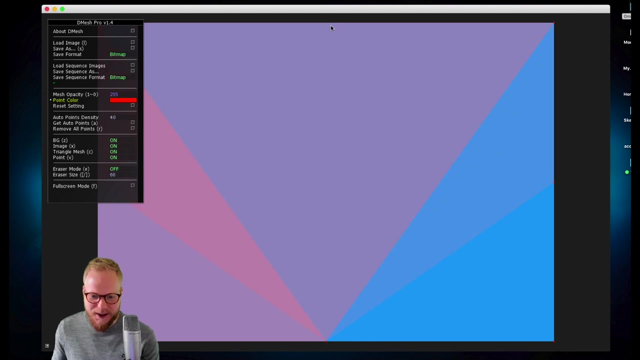 my mobile app or something. I'm going to export it as a JPEG, go back to D mesh and I'm going to load an image. quite old school, vintage interface, you can tell right, But nevertheless you know you can't overlook it And if I load this thing as you can see, it automatically creates me. 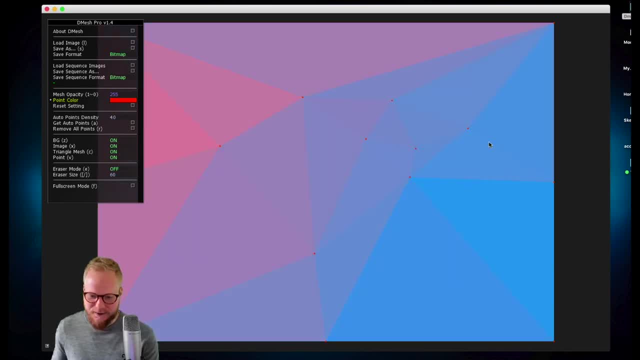 fractals, And then I can add new points for it to make it more fractalized and more diamondy per se. That's pretty cool, isn't it? Now, here you can also check the color of the pointer, So you can make it white, you can actually disable it, you can reduce the opacity. 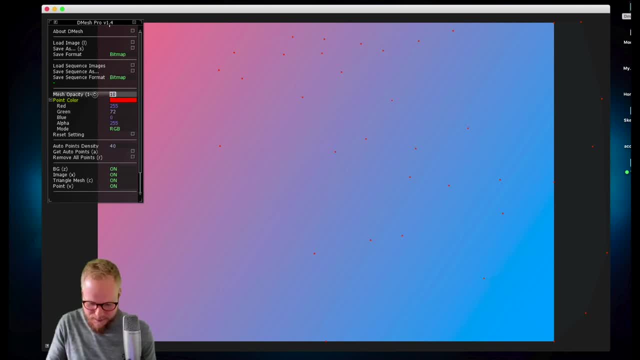 So it's all quiet, neat. But let's say, if I make it 300, you can see the outlines. point density you can increase it, But once you start adding the points, you're going to see that it fractalize your image. You can also preview it against different backgrounds. 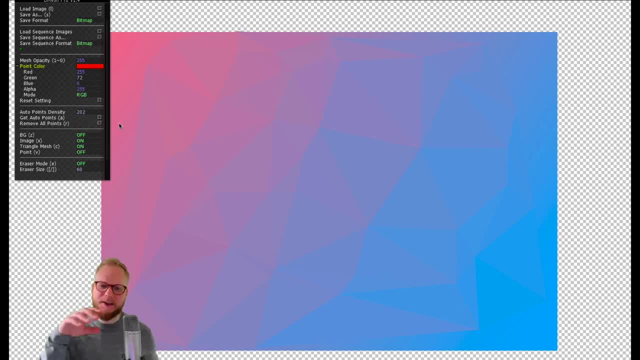 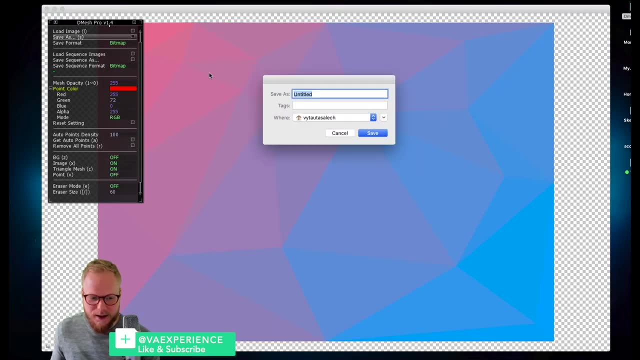 But, as you can see, that's that's how you do it basically And it's just because it's such a subtle gradient- And maybe that's the background you're looking for- You can also save it really quickly And, as you can see, it made this type of background which I can edit and do other things. 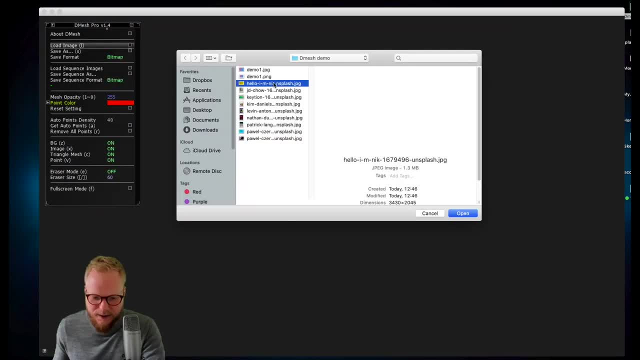 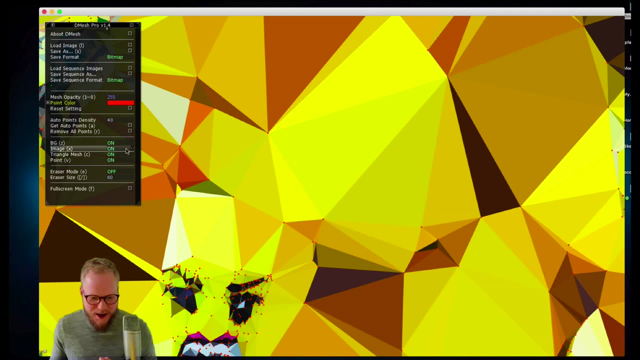 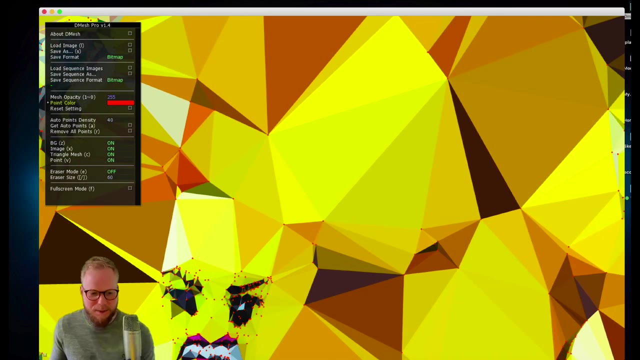 with it. And so if I open a new image and let's see, let's check something a bit different, So I'm opening Legos automatically, you're going to see that it creates much more powerful thing. and it's because the image is so large it doesn't even fit, but you can see the application of it. 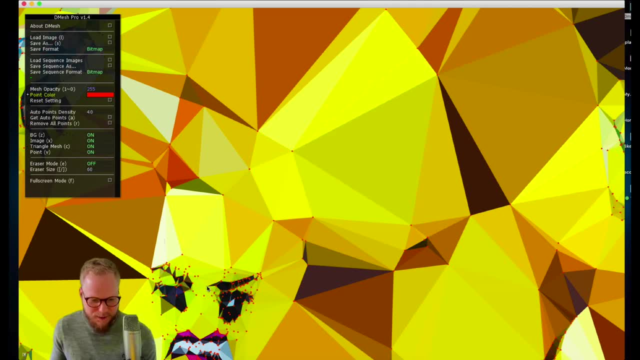 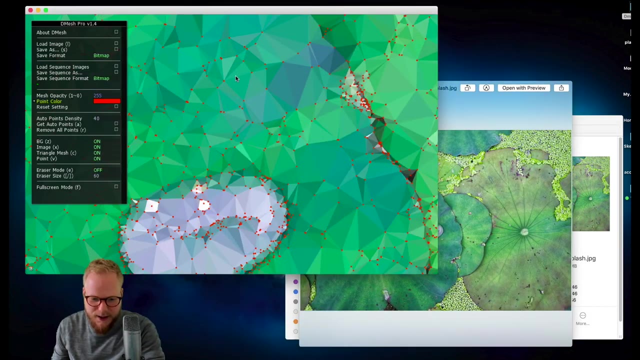 and how cool that could look like, And you can edit all those points. you can disable the points as well. Let's say, if I disable it, you can have this type of background And you can, of course, play with it too. And you can see exactly that I'm taking this image and I'm putting into D mesh. 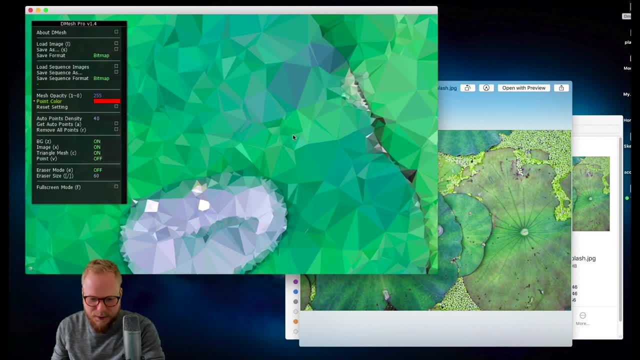 And that's the result. So let me just take those points out. But, as you can see, the more contrast there is between the colors, the more contrast there is between the colors, the more contrast there is when you clip them And then, as you can see, the more fractal it gets And if I, let's say, would